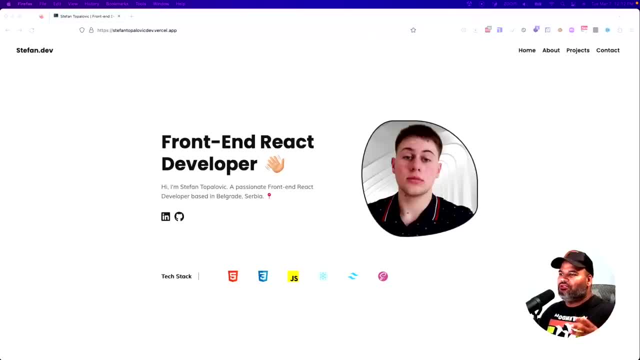 of hard. they're more like medium positions than junior. they want us to be the next elon musk. do you have some tips for me to find a remote job from the us um where it'll be okay to work with someone outside in the us? i'll send you my cv, so maybe you have some tips. 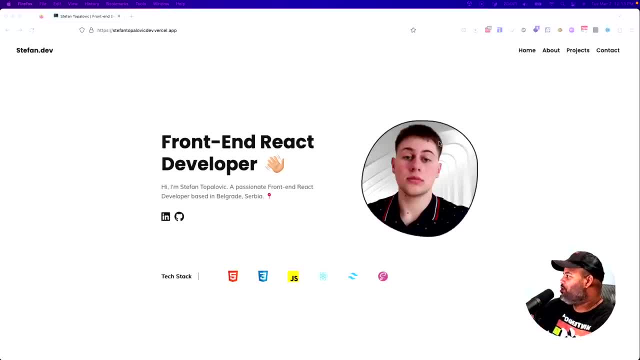 for it. okay, cool. so again, this is portfolio right here and i'm gonna be honest with you guys. yes, he just started a few days ago. okay, as far as, like, hey, he puts his portfolio up. but i'm gonna be honest with you, i think he's ready to go. okay, i will give this a 9.5 out of 10. 10, like i said. 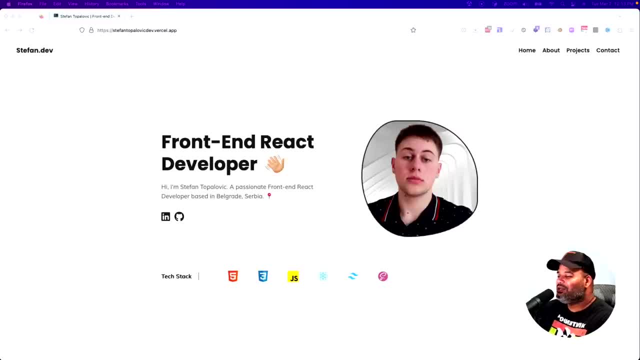 uh, most likely, and it's because it's a really good portfolio. okay, so again, uh, let's go in. it's very simple portfolio, know, fancy animations, nothing too crazy, okay. front end react developer: stefan topolovic: uh, passion. front end react developer based in bagrade: uh, servia. okay, tech stack html: css, right, javascript. 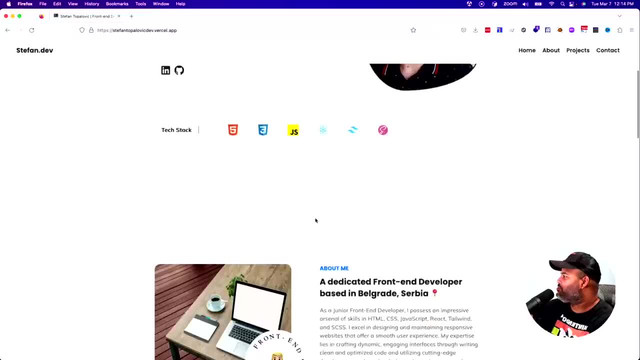 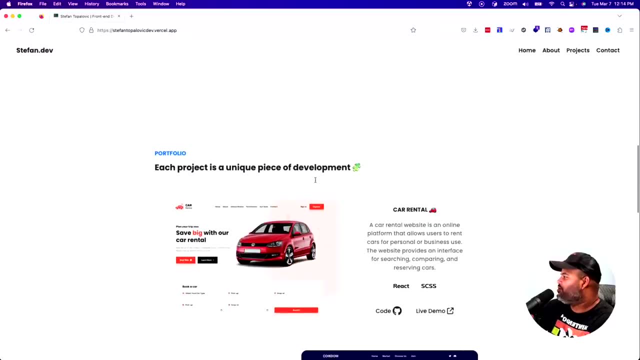 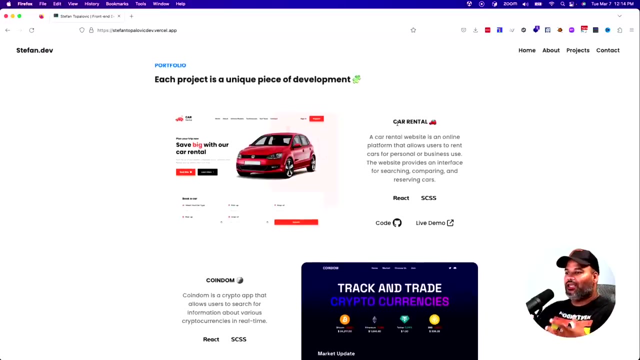 react: tailwind sas- all right, cool. so in here he has his about section. very nice, okay. each project is a unique piece of development. so in here what i really like about this portfolio is that he has like real applications that a business can see themselves and say, okay, he can come work here he. 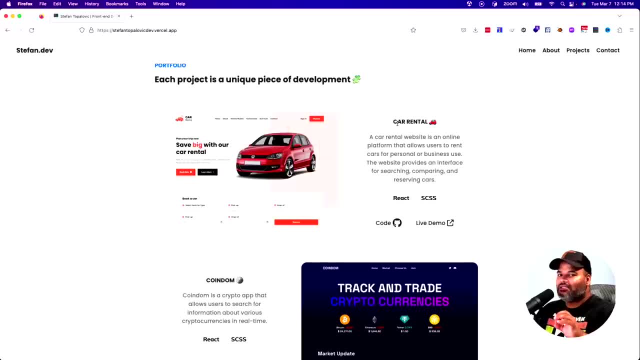 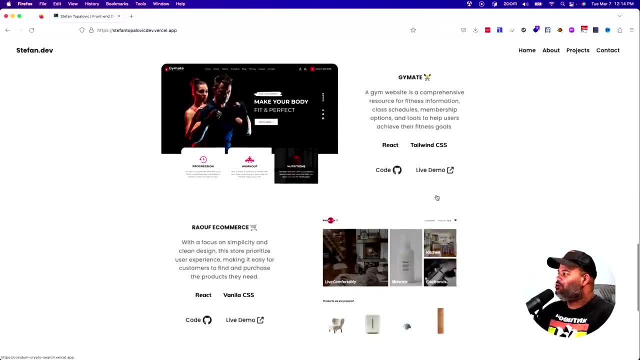 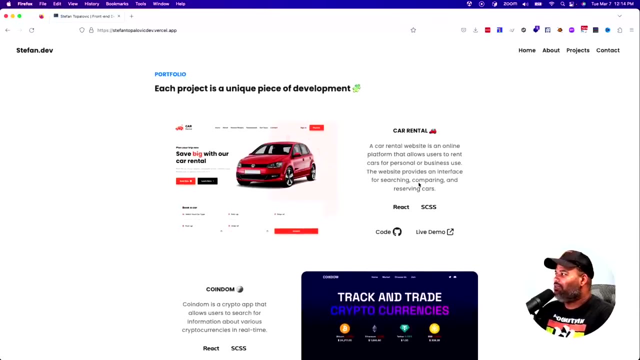 can do this type of work. here and again, everything is like pixel perfect. everything just seems very, very polished. um, you're not gonna find no random a to-do app, no web api app, no little javascript snake game like. everything here is pretty much like: hey, uh, this is something for a business which is 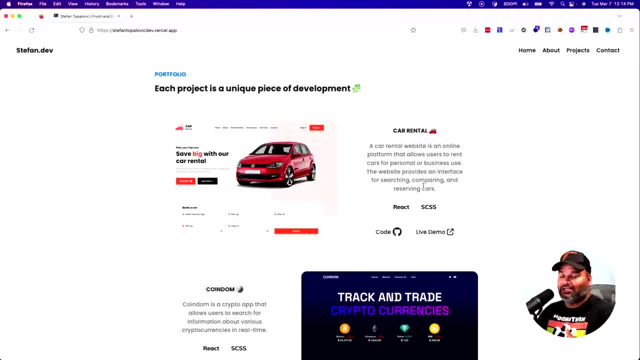 something that i always recommend to every single one of you guys. this is how you actually get higher. show that you can actually do work for the type of positions that you are going for. stop going in and just putting in random projects just to fill it up. people don't care about that. you did 30 tutorials on youtube, right? don't put those projects in there. 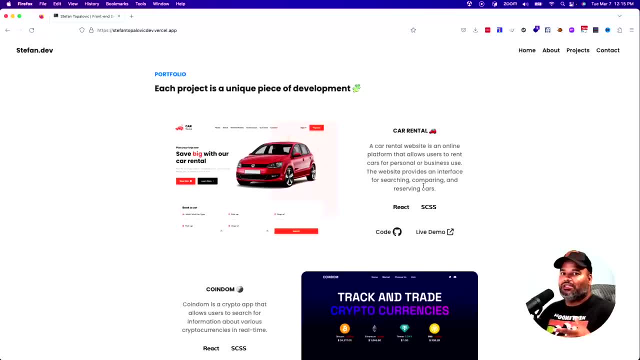 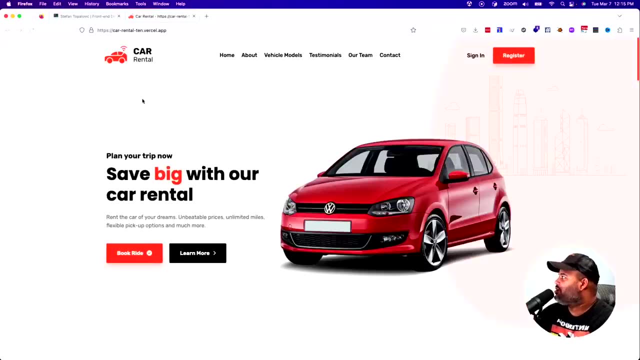 what you want to do is you want to go in and build solid projects that a business can say, okay, this is a business that you're going to go in and build solid projects that a business can say, okay, this guy's ready to go, all right. so let's take a look at this first project over here. uh, this is a car. 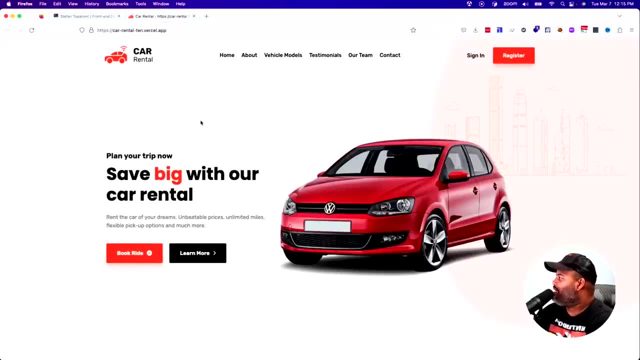 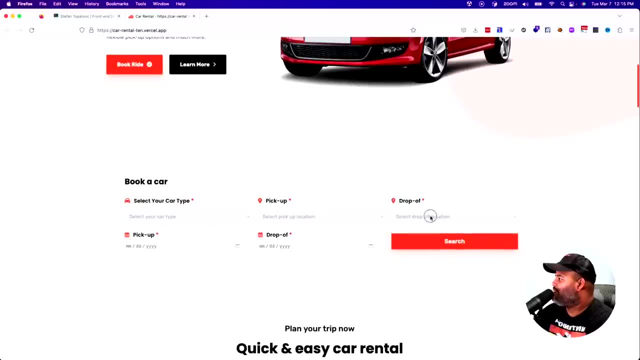 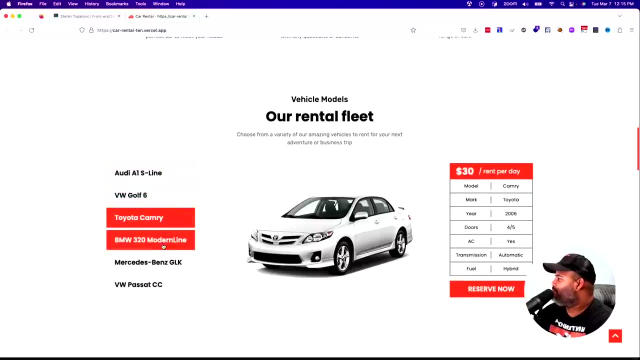 rental service: okay, the design is very nice, everything about it is very good. like i have, um you know, any complaints about this at all. right, very nice, okay. uh, rental fleets: okay, he has the different rental fleets. as you can see, everything changes: the different pricing, the different models. so again, he's taking 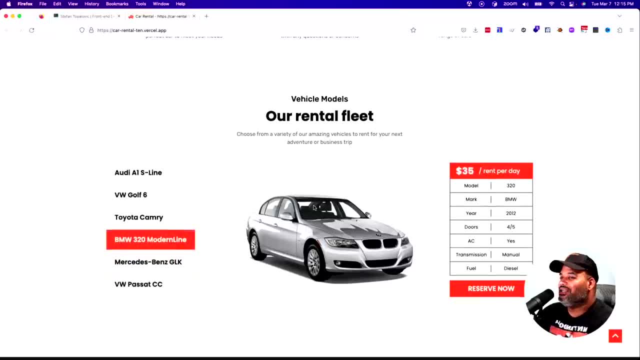 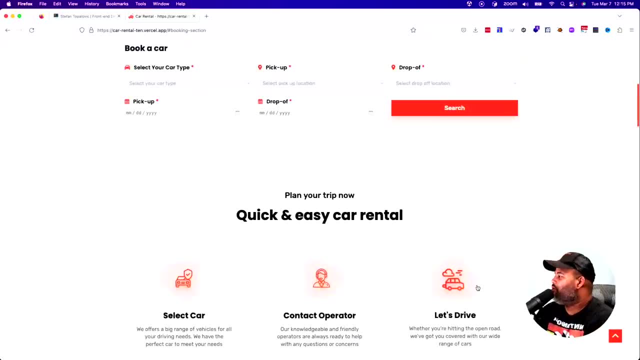 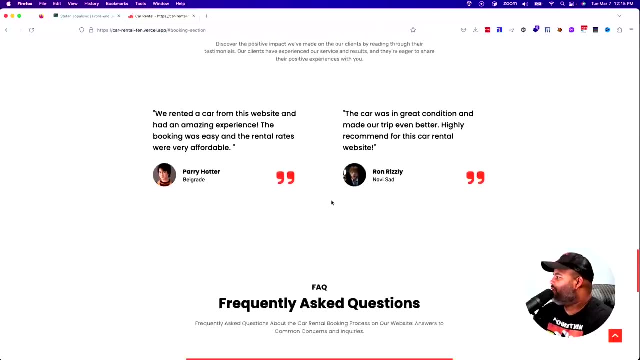 his time to go in and make everything interactive. he could have easily just stopped right there and say, hey, this is the landing page, ta-da right. but he's actually making everything you know uh work. so again, very nice. okay, let's see here again. the design is very good, it's really helping. 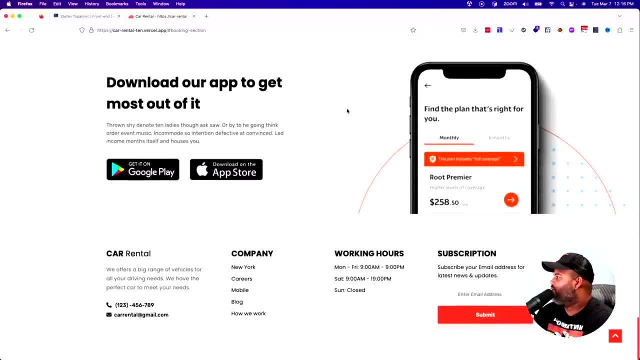 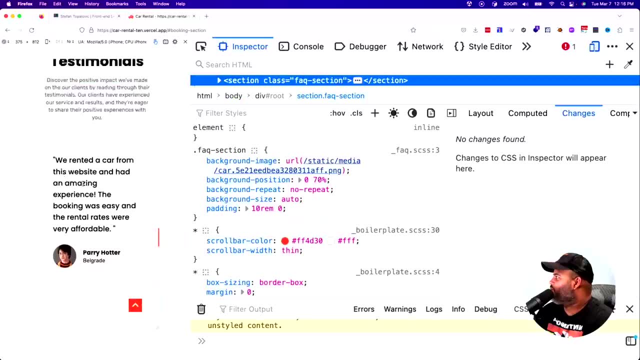 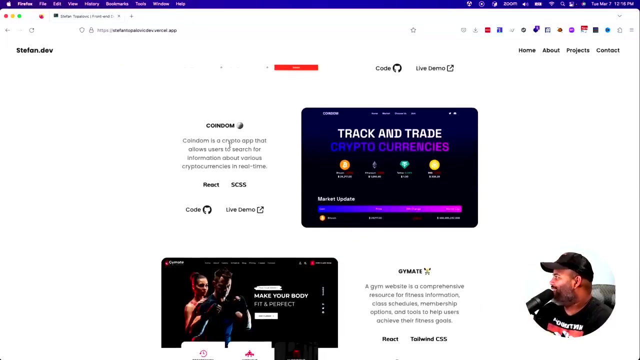 him out. okay, everything works. and let me see if i open up my inspect element. make sure this thing is responsive, looks good. yes, sir, okay, your boy's not playing no games. okay, very nice. okay, let's go to the next one. we got a coin dump. you got to be careful with this. 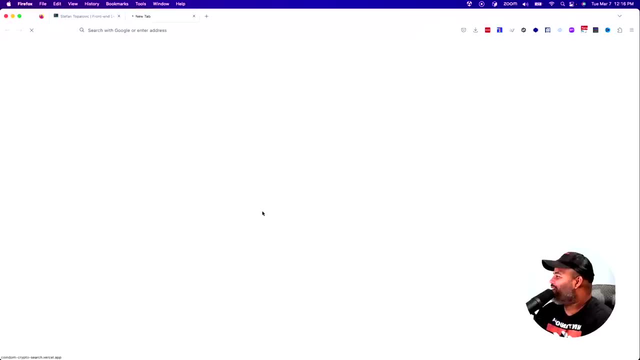 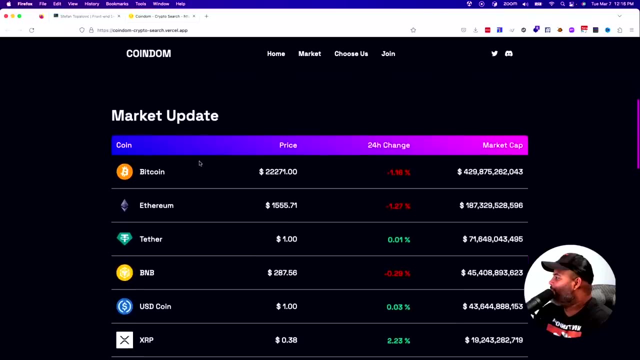 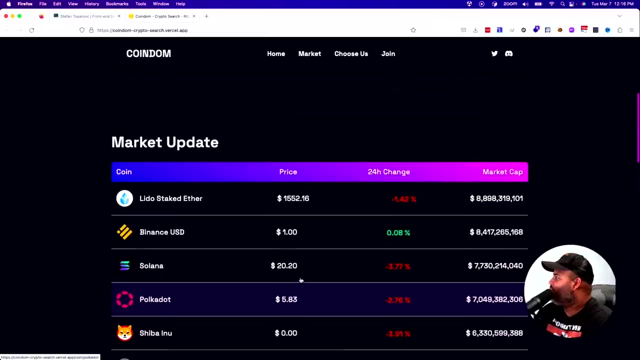 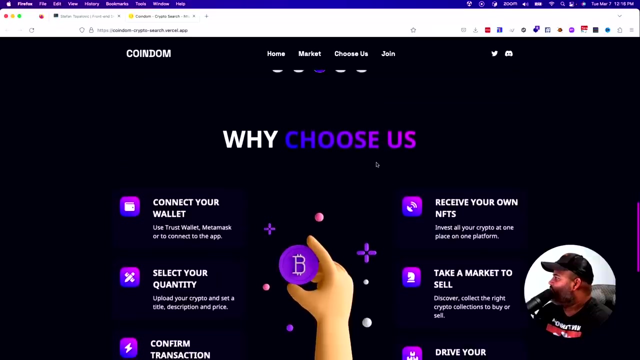 these names right, so it's coined them right. i almost said something else, uh, but again landing page. very nice, nice little animations, okay. again in here he's showing us like he can work with different apis, so this is actually pretty good. okay, there we go. let's change in the different coins. okay, why choose us? connect your wallet. 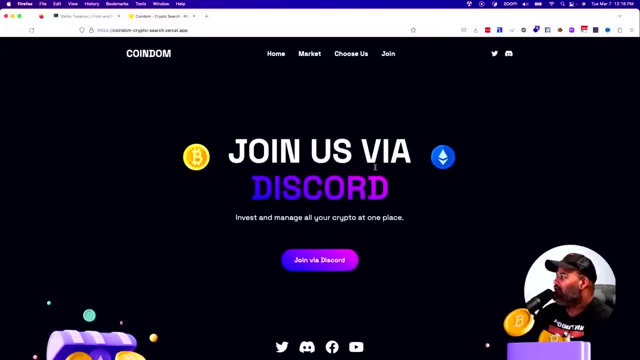 again, the design of it. it's really really good and this is something that you guys got to keep in mind: if you show people that you can build something with a good design, even if you didn't build the design yourself. you could find designs online from the website. you can find designs online. 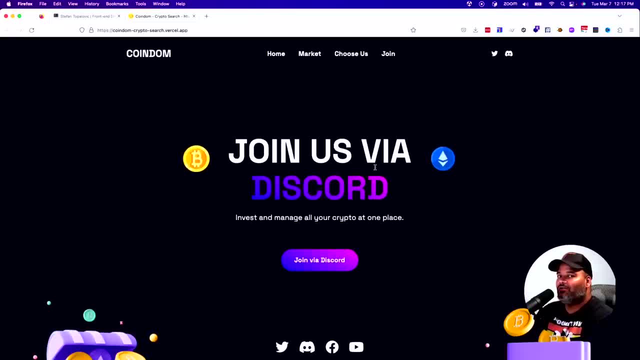 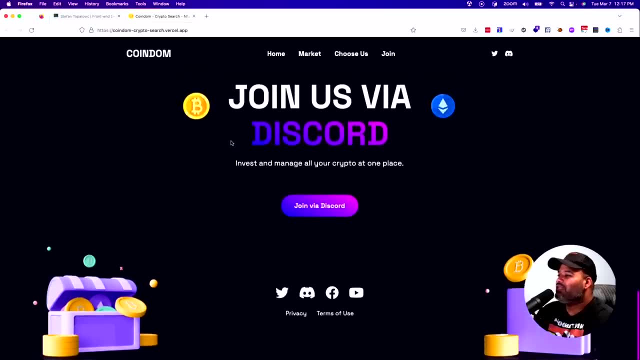 dribble to. you know other websites that already have beautiful designs and then you go and recreate them, right? if you're able to do that, then guess what? it's just going to show them that, no matter what they throw at you, you can actually go and build it, and if they give you a really good 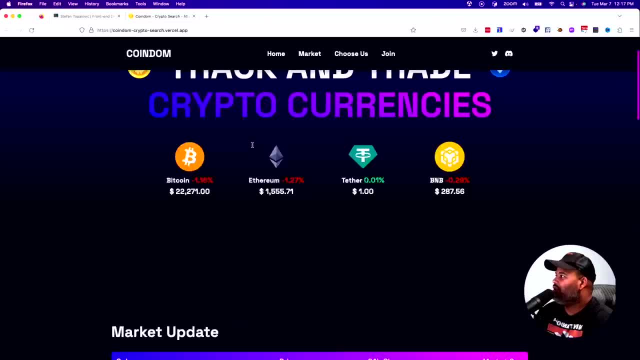 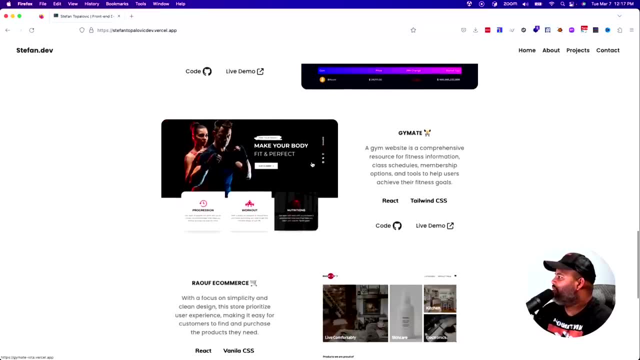 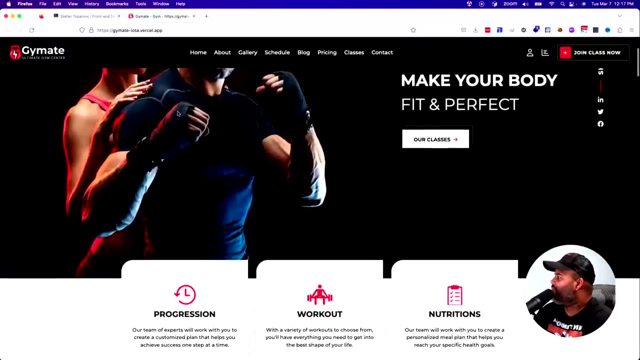 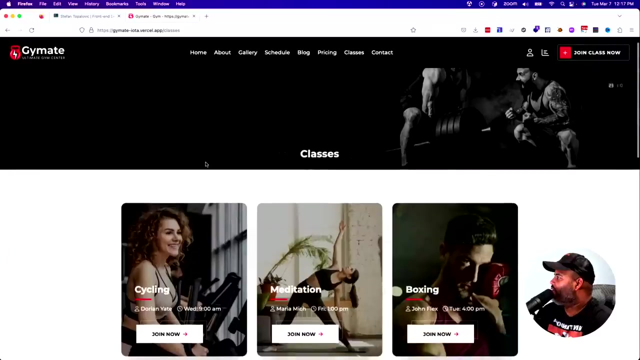 quality design. you can go in and execute it and make it into a real website and a web application. okay, the next one we have right here is gym eight or gym mate, so click over here. very nice, okay, nice hover effect. okay, it actually goes in. it takes you to the different classes. so this is. 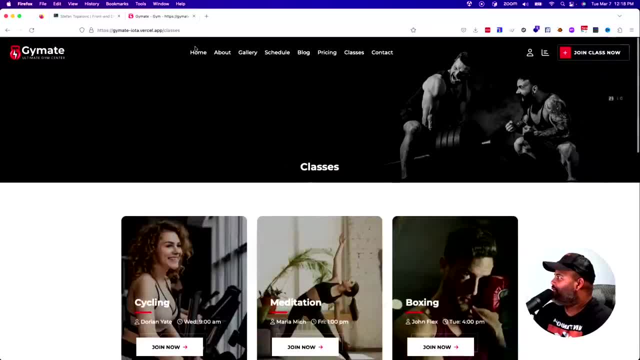 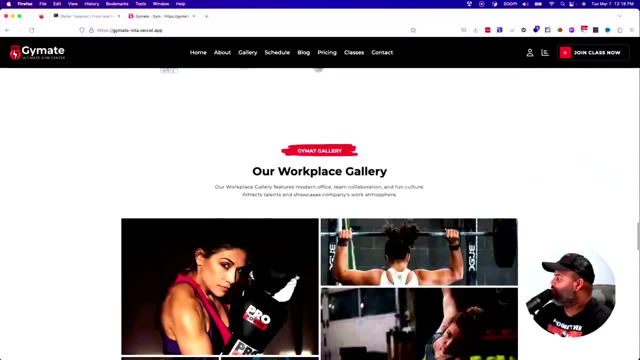 like the little details going the extra mile. okay, sometimes people just go in and build a landing page and don't even have to wait to solve the training. they just go in and build it and get, even try to do the rest of the pages. so again he's showing you that he could build a full website. 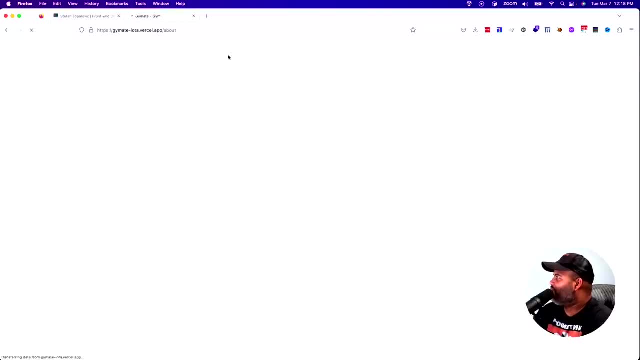 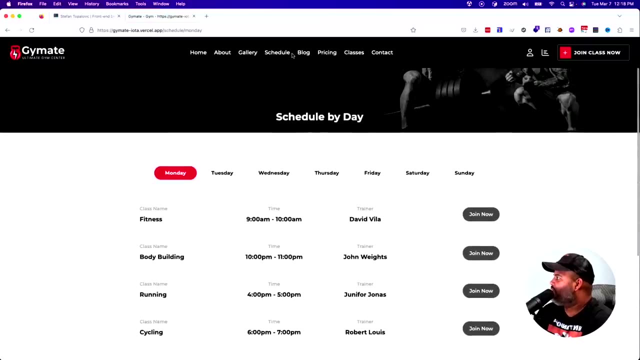 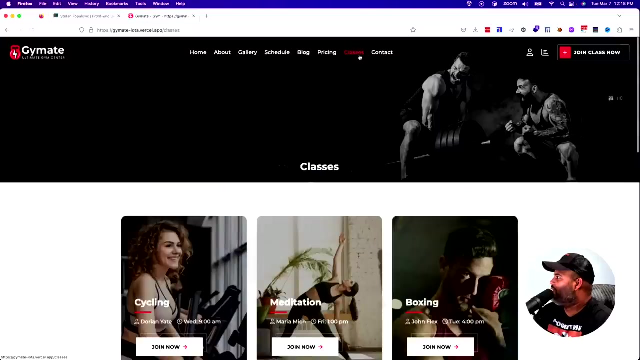 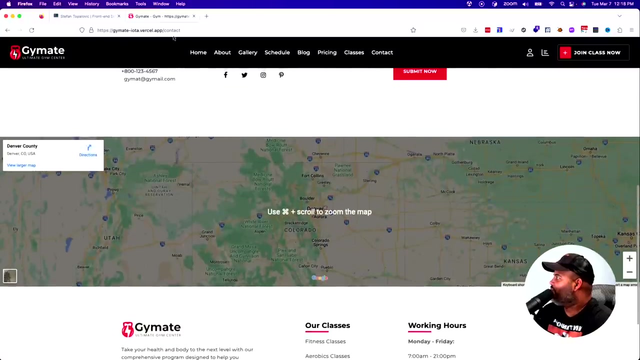 all he needs is the design and he can go and build it. so again, very nice. got the about page. got the gallery page. got the schedule page. okay, got the blog. got the pricing: okay, got the different classes over here. got the contact page. so, yes, you can go and build you a full. 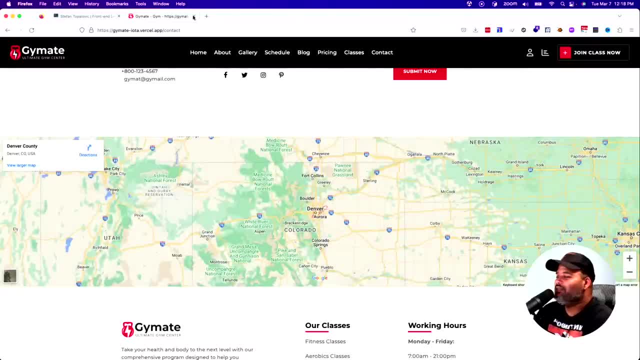 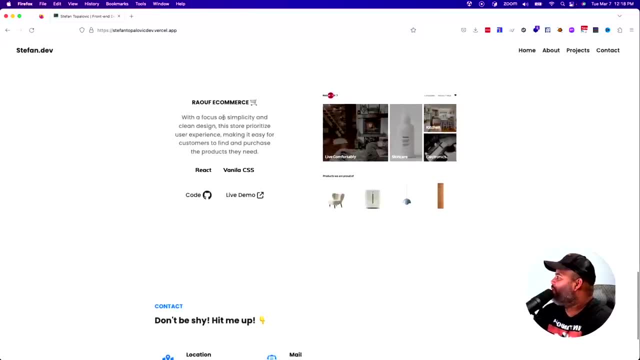 site. if you give him the design again, he's a front-end developer. all right, let's go to the next one in here we have rough e-commerce. so basically the focus: simplicity, clean design. the store: prioritize the user experiences, make it easy for customers to find a purchase. 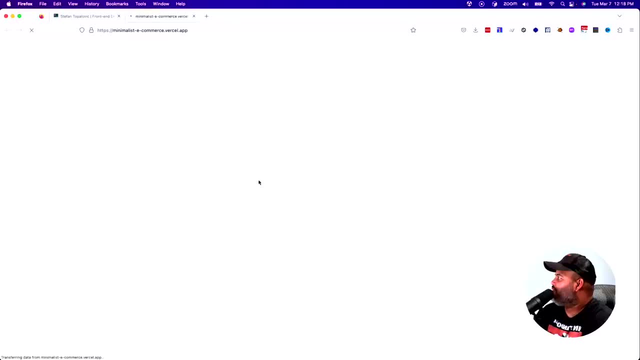 product and then you can go and build a full site. so again, he's showing you that he could build a product react with an lcss. that's what he used in here. okay, pretty straightforward. okay, let's see. okay, he does have a product page. all of this is working. click add to cart. the cart. 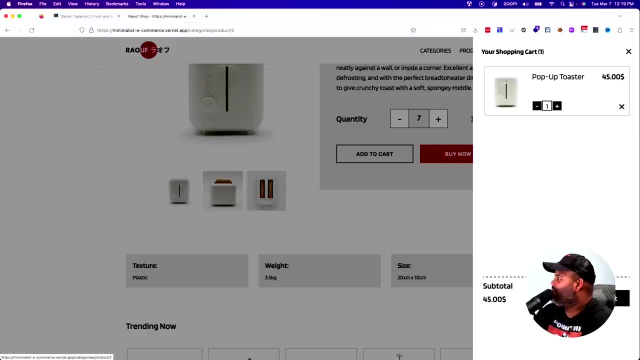 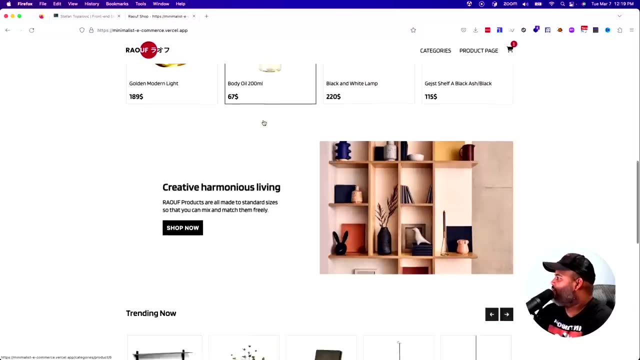 is actually working. there you go, let me see. maybe it goes to the checkout. it'll be nice if we would have disconnected to stripe, okay, but again, very nice design, very nice website. very nice website, very nice product. react with an lcss- that's what he used in here. okay, pretty. 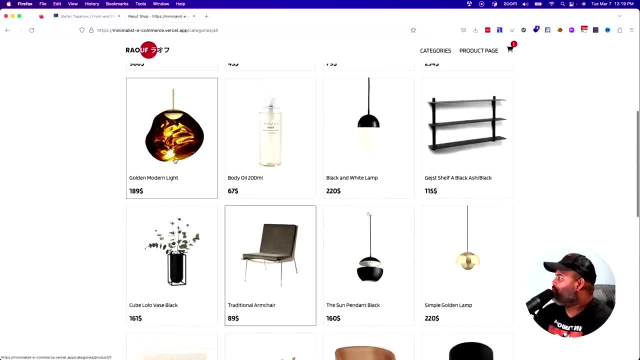 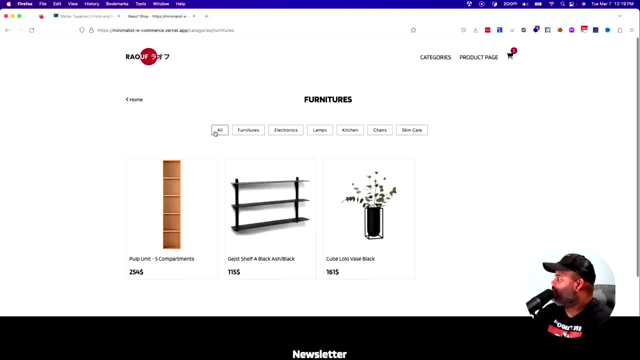 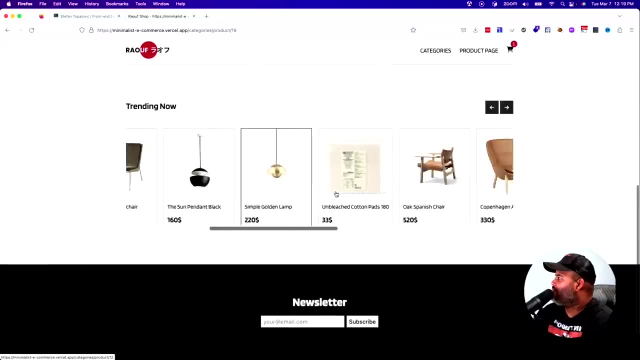 site, uh, pretty much showing all of the skills that he has as a front-end developer, uh, which is really good. you see, everything here is very polished, everything works, all the filtering systems okay, and again you have the product pages right here. you have a trending now section, so yeah. 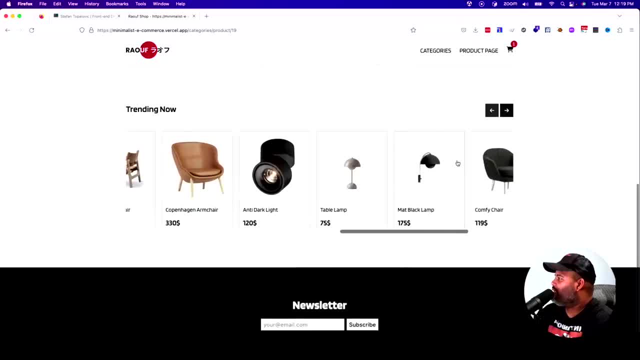 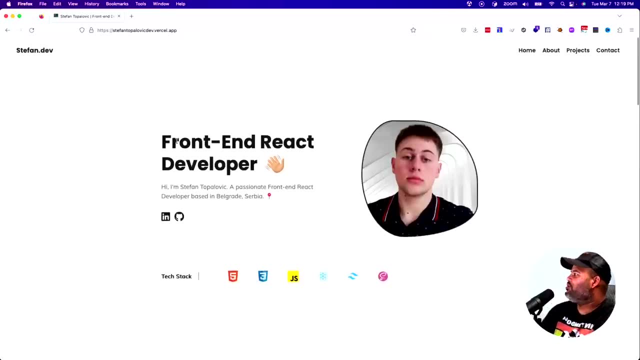 you know there's no complaints in here. i'll be honest with you guys. all of those projects look legit, okay. so again, shout out to your boy: stefan, this is what you call a really good portfolio. guys, again, if you want to get to a level like this, definitely check out codingfacecom for those. 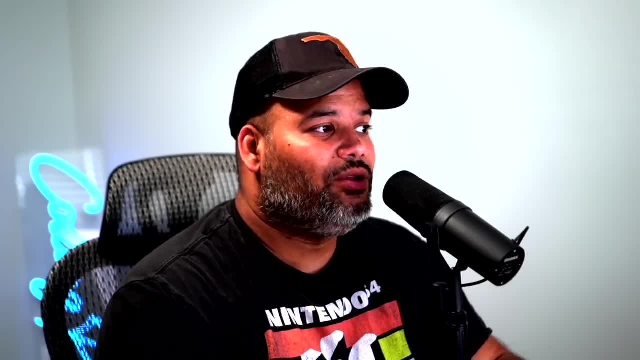 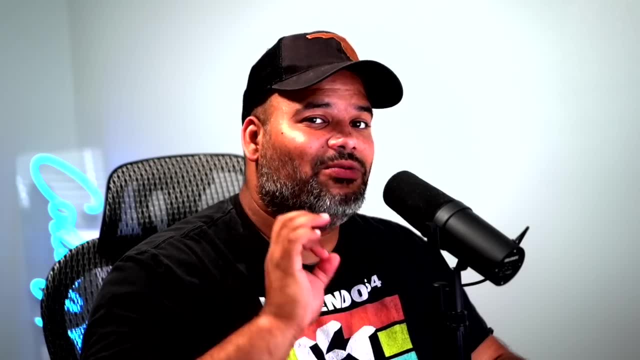 of you guys that don't know. we do teach people how to code. doesn't matter what level you're at, we can help you out. if you are a completely beginner, like you, have no knowledge of programming, we can help you get to a point, just like stefan. 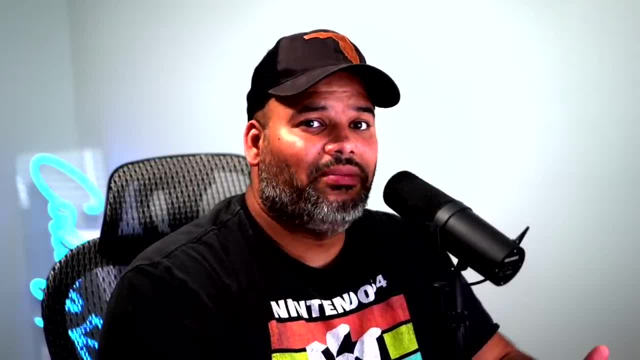 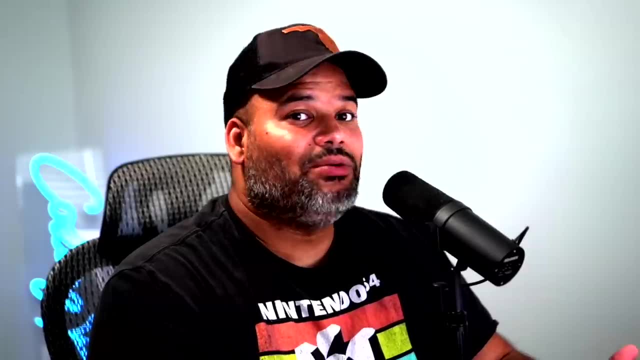 so again, shout out to him: his portfolio is looking great. it's only a matter of time, uh, from you know from now to when he's gonna get hired. now my advice that i will tell him right, because he's outside of the us. sometimes it's a little bit difficult for people to find jobs in the us. 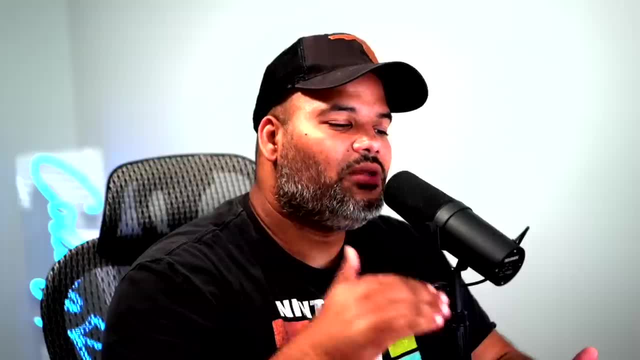 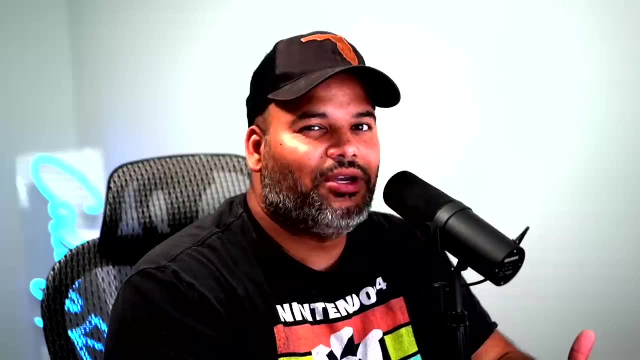 market right, but what you want to do is you want to start looking into other type of uh technologies, or you know frameworks or libraries, you know pretty much just uh different ways that you could get to a level like this. so again, shout out to him: his portfolio is looking great. it's only a matter of time. 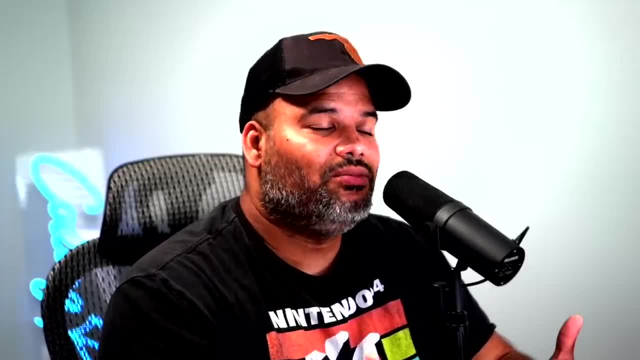 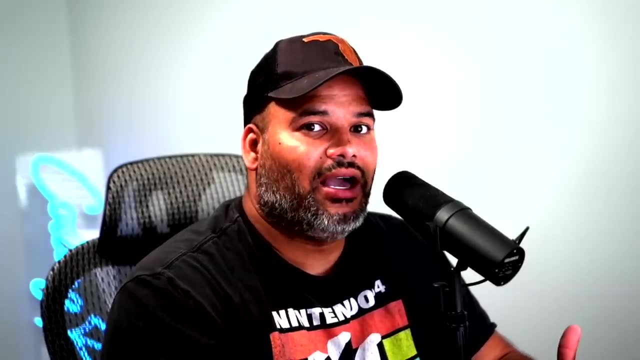 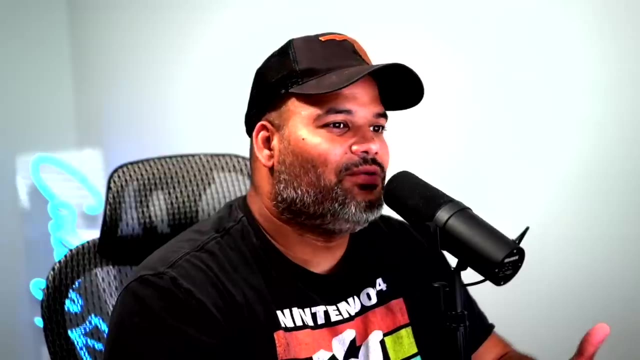 get in um again. react is very popular, so you have a leg up because you have a really polished portfolio. i will also recommend that you go and check out typescript and also to check out angular. okay, now you might say: well, joe, i love react, i'm a react developer. but this is what i'm gonna tell. 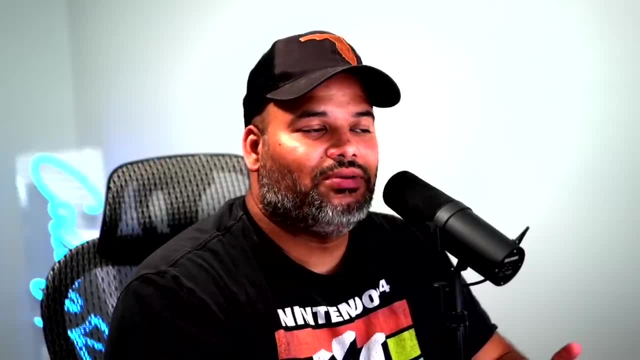 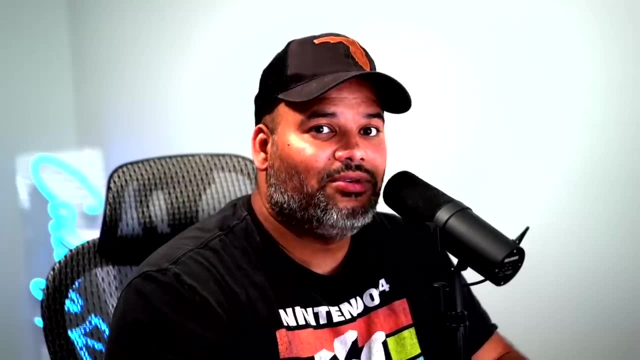 you right, hear me out if you want to find some opportunities right and you're seeing that you're applying to jobs. you're applying to jobs and you're not getting the responses that you want. you're not getting the that you deserve. guess what? try to get in a different way now. a lot of people are paying. 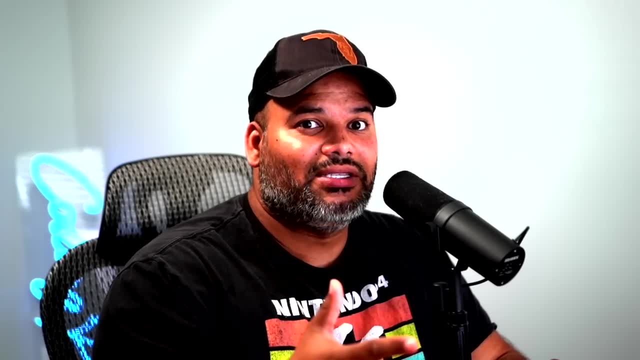 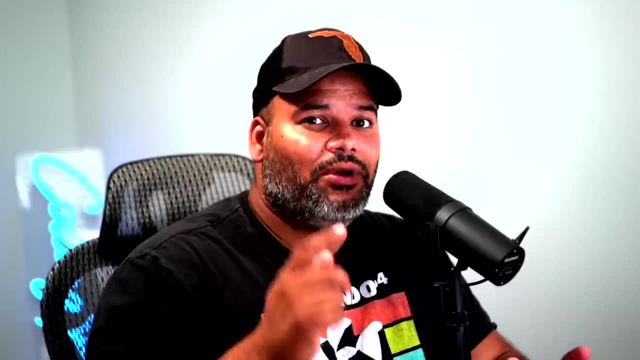 attention to angular. they're not really paying attention to the opportunities that's there because they kind of don't want to do it. everybody wants to do react and that's fine. you could do react on the side. you could do it on your own projects. but if you want to get paid, look for. 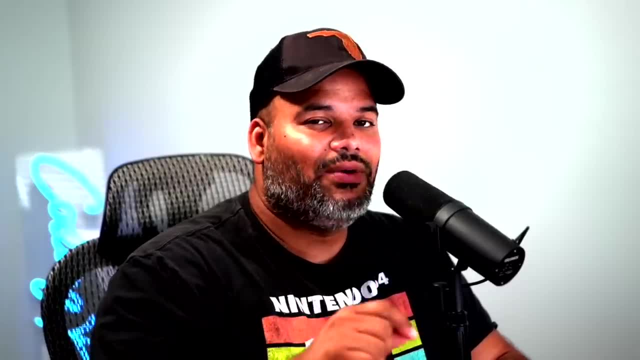 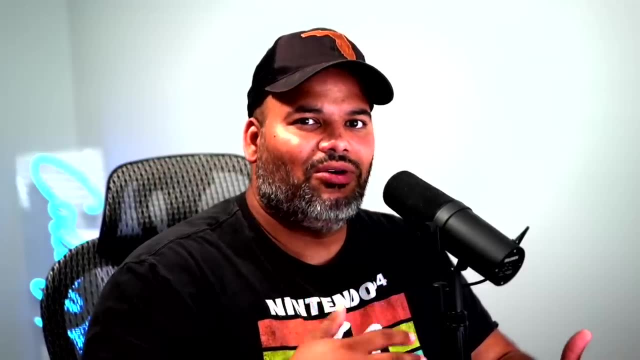 ways to get into the industry quickly. okay, angular, right now no one's paying attention to it. so if you go in and go over angular, maybe you know get a online course. or here on codingfacecom, when you go over the angular course, you could pick it up like this: it's: super quickly, right, and then from there, just build one more project in angular just to show your diversity, and then apply for all of those angular positions from servia. you can definitely get a job as an angular developer for sure. now, of course, you're going to continue applying as a react. 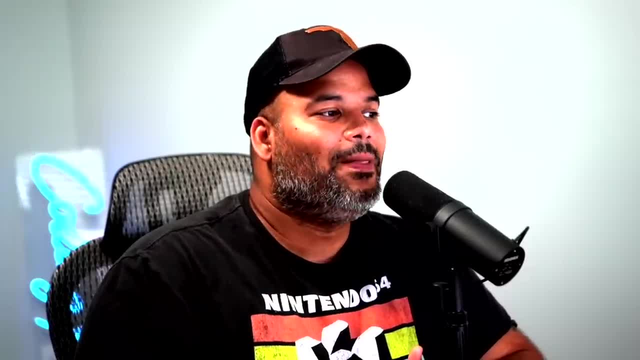 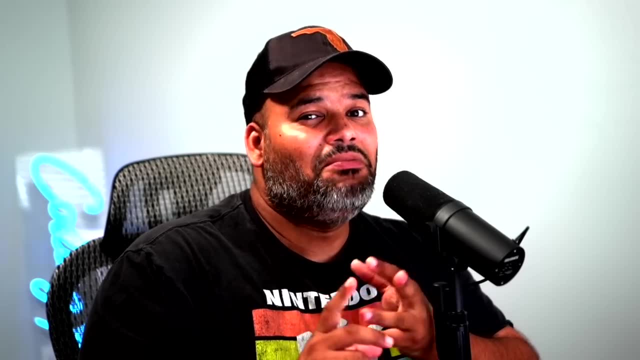 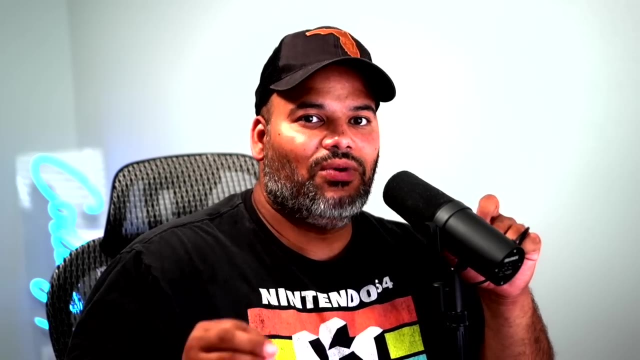 developer. i'm not saying to stop applying for those roles too, but you want to go in and start adding some more projects, maybe some angular, maybe some Shopify and maybe even a WordPress site- And again, I know how people feel about WordPress. but when you're outside of the US, what you care about is this: Okay, You want to. 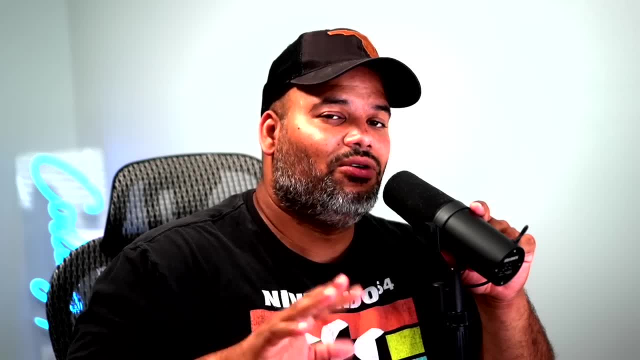 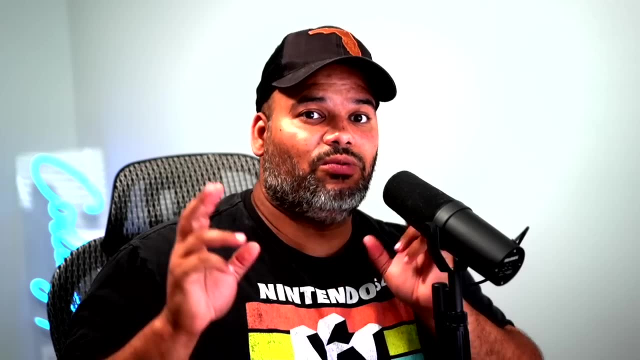 get your money Okay, And there's a lot of opportunities there. Don't leave those opportunities on the table Now. you could stay at home and wait, you know, six months a year So you find the right front end position as a react developer. or you could say: let me start working now. 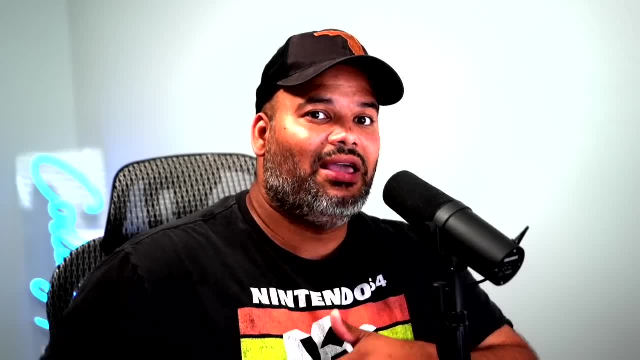 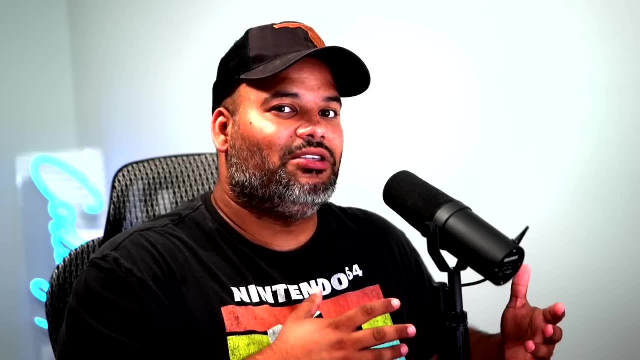 builds an experience. And guess what, When you go in and apply as a react developer now, you got six months of experience, a year of experience right Using web development technologies that are adjacent to it, Like again and angular and WordPress. So keep that in mind. 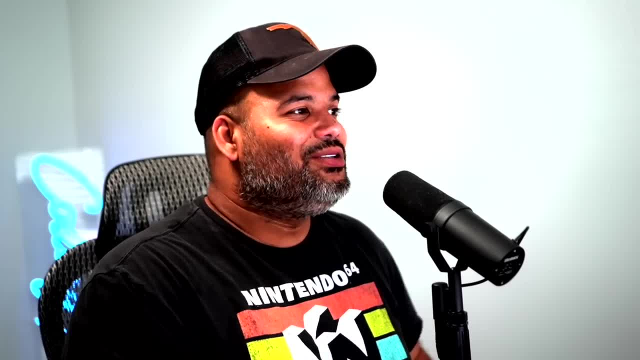 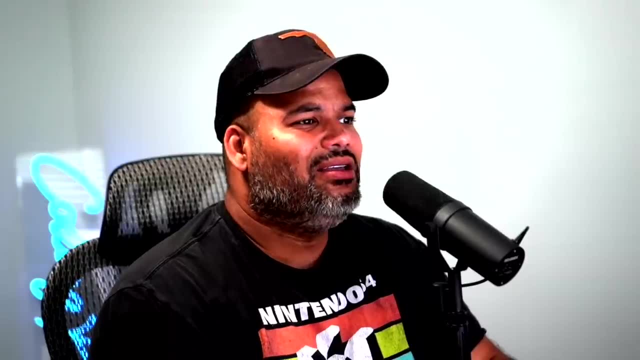 you know, play chess, not checkers. All right guys. So again guys, like I said, if you guys want to go and learn how to code, check out coding phasecom. It don't cost nothing to go check out. 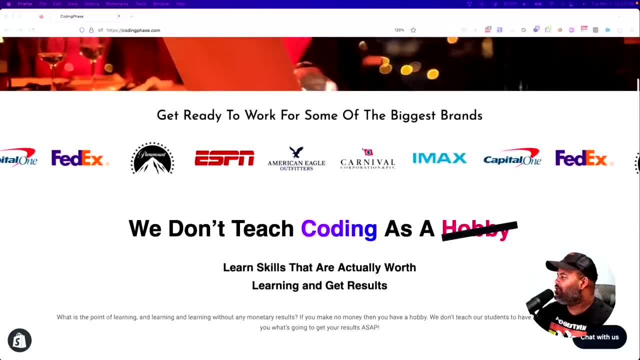 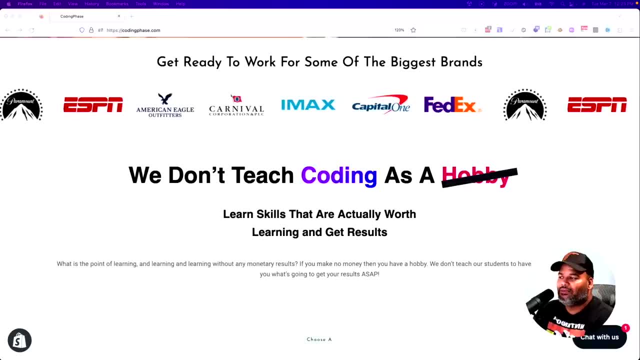 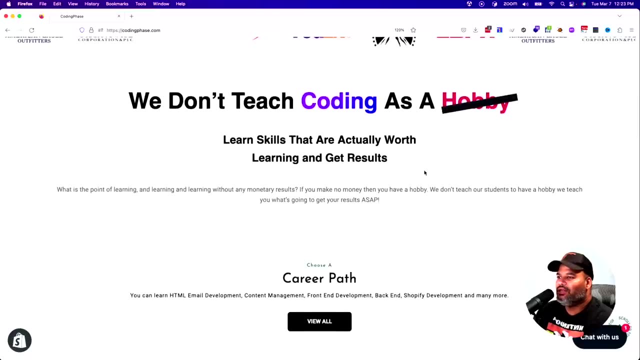 the website literally. You know we teach coding not as a hobby but for a goal: to either make money as a developer independently or to start getting a job Okay. So again, the whole goal here is to get you guys into your first position, And that's what we do at coding phasecom. You can go in check out some. 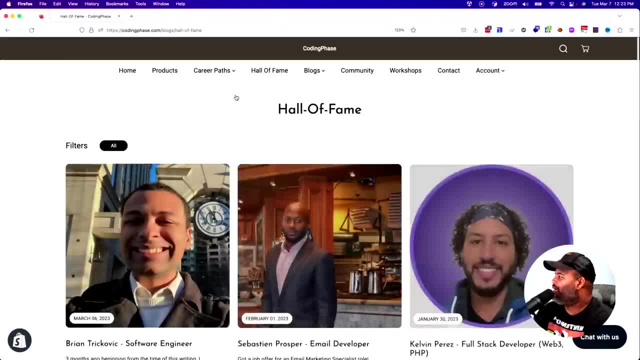 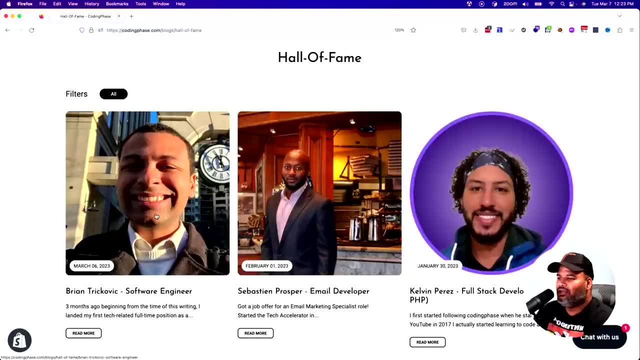 of the stories from the hall of fame. Again, shout out to Brian, the latest member that we added to the hall of fame. hire as a software engineer. been killing it on the past few months. And yeah, shout out to us. 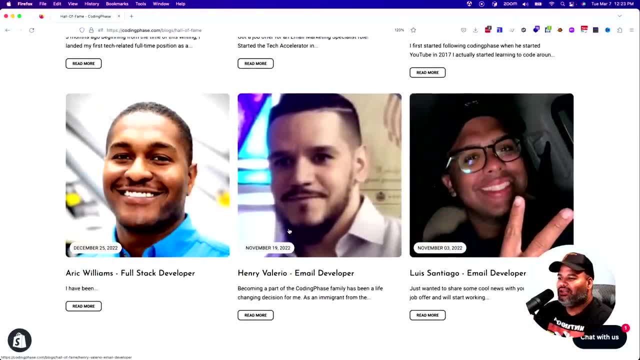 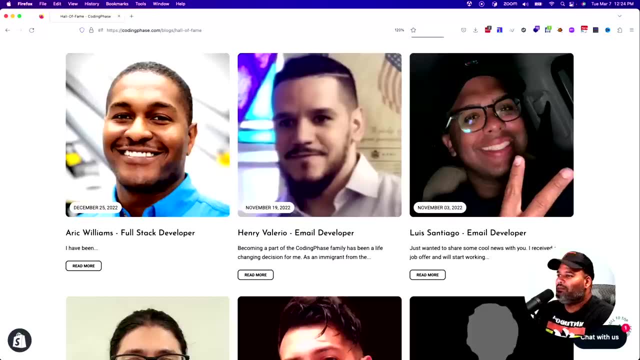 Sebastian, Kevin Paris, right, Eric Williams, Aaron Valerio and all the other guys that we are going to be adding to the hall of fame in the near future. But yeah, like I said, check out the platform and I'll see you guys later. It's your boy, Joe. back at it again. 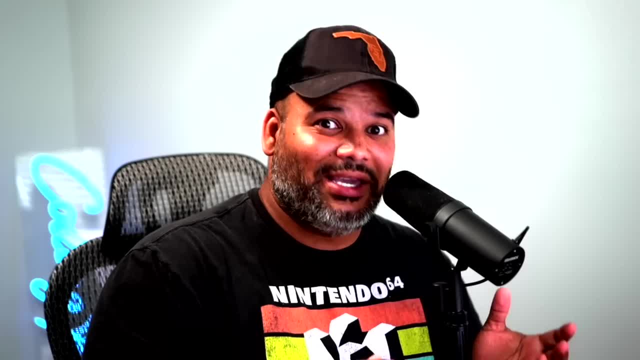 coding phasecom. Stefan, congratulations, You have an amazing portfolio. See you guys later. Peace. 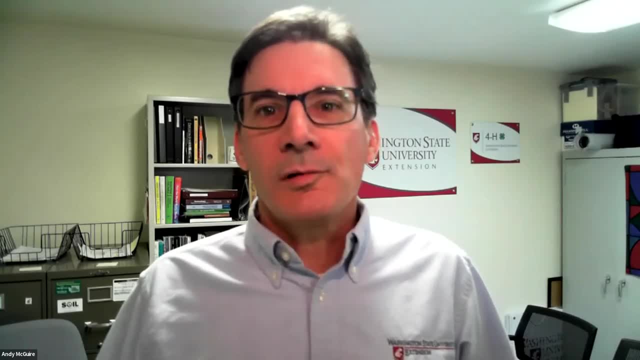 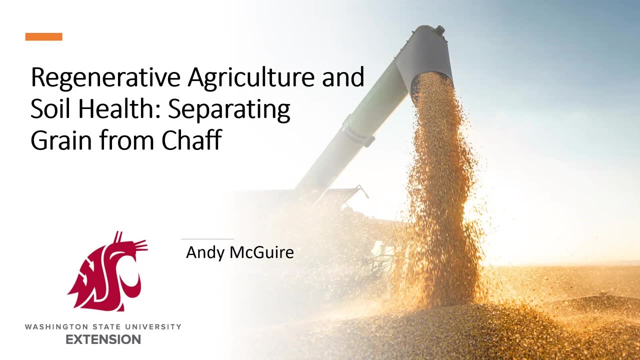 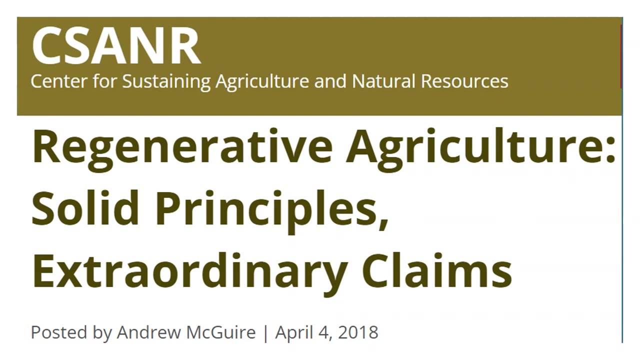 Let me share my screen here, All right? Well, I've got a lot to cover, so I'm just going to dive right into it. Yeah, back in April of 2018, I wrote this piece about regenerative agriculture. you see here, and: